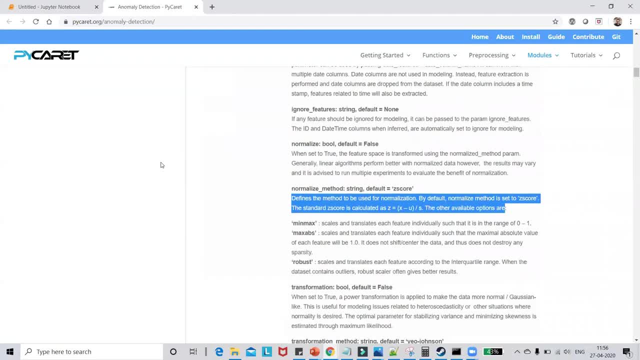 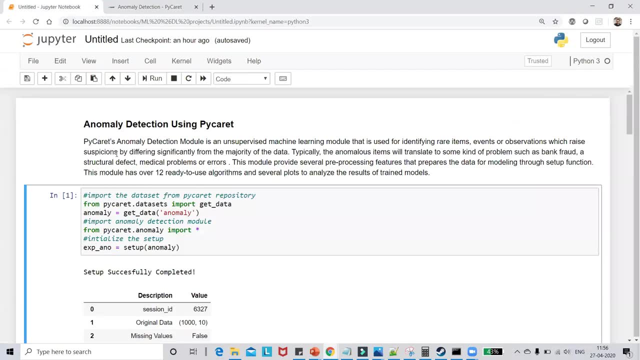 I'll also be giving you this particular URL so that you can refer what are the different different anomaly techniques that this PyCaret open source library also use. So let us go ahead Now. first of all, just to understand what is the anomaly detection Guys PyCaret. 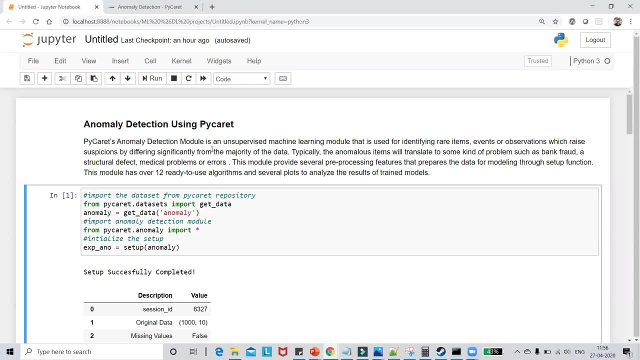 is an anomaly detection module. It is basically a module in this particular case- and you know, anomaly detection is a use case itself, right, It is an unsupervised machine learning module that is used for identifying rare items, events or observations which raise suspicions by 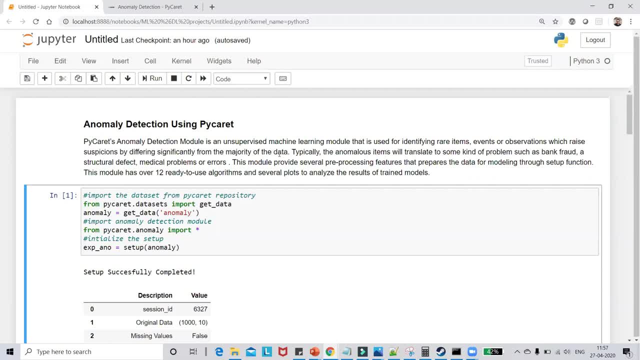 different significantly from the majority of the data. The best example is bank fraud, structural defect, medical problems or different kinds of errors. This anomaly detection algorithm is heavily used in banking industries, you know, in banking stuff, whereas in manufacturing industries and, if I take some more examples, right in network trafficking traffic companies. 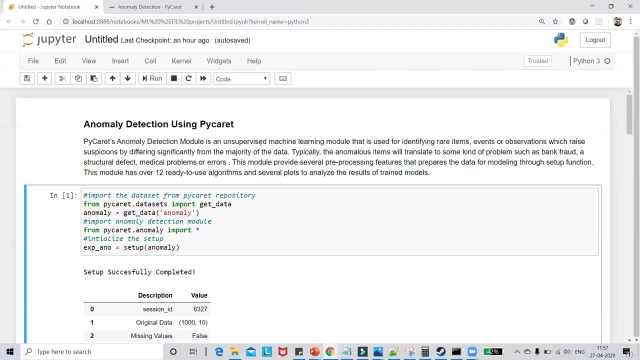 also right. So they are used in many such use cases. Now, if I talk about banking domain, right, you'll be able to find out that there are a lot of fraud transactions there. that is actually happening because there will be so many transactions And out of those, 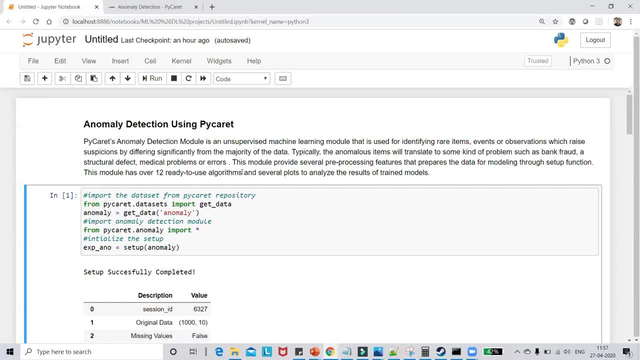 transactions. how do you determine the fraud transaction? That is pretty much important, right In the case of network traffic. you know companies where they are actually having a huge product, like routing products, or where they see a lot of traffic coming through their 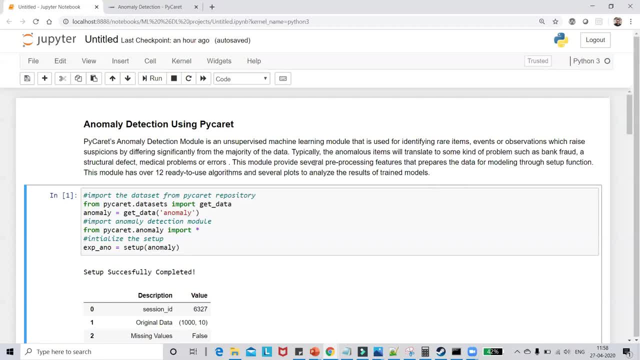 particular websites through various means right At that time, in order to determine from those traffic which is anomaly, basically which is a fraud one, or is that traffic coming from a different source, like kind of a hacking code, Kind of stuff, right? So it will actually help you to do this kind of anomaly detection. 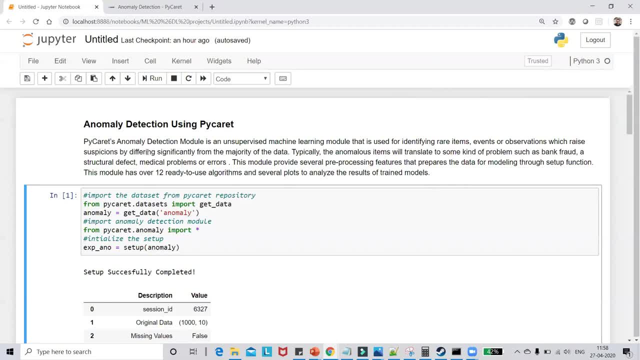 It is a wonderful use case, guys, And again, remember this is an unsupervised machine learning technique. you know you will be getting the data like you will be getting all the transaction data, And out of those transaction data you need to just pick the. 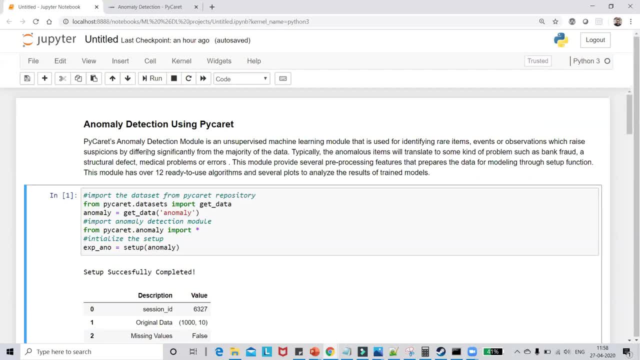 fraud transaction data And again, just understand if it is unsupervised machine learning, it is very, very difficult to actually do that particular work. Now PyCaret again has come up with a wonderful open source. this particular this is an open source library which will help you to. 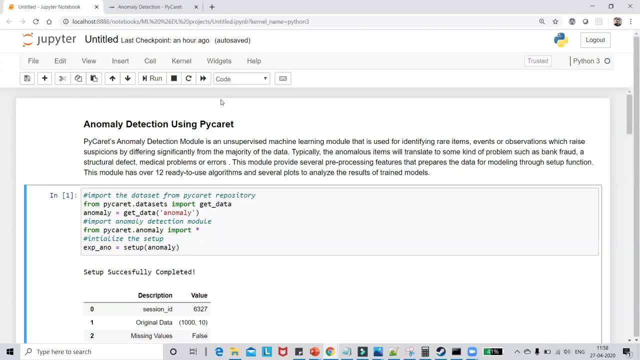 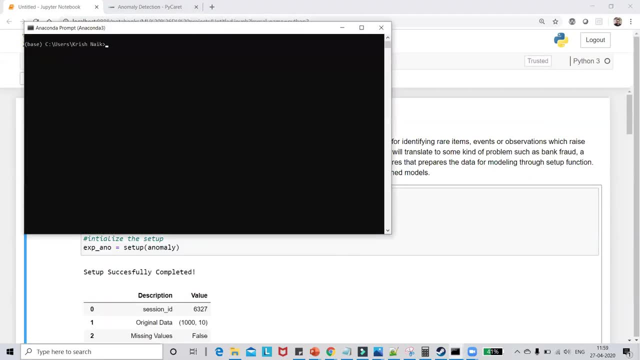 do that right. So first of all, in order to start with guys, make sure that you create, go to your anaconda prompt right And just create a new environment. Suppose I have actually created an environment called as NLP, right? So inside this particular environment and 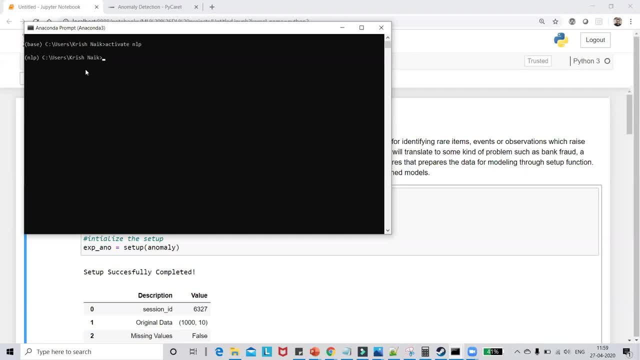 make sure that if you're installing PyCaret first of all, you make or create a new environment. don't do it in base. it is always a good thing. You should practice that whenever you start any project. it is better that you create. 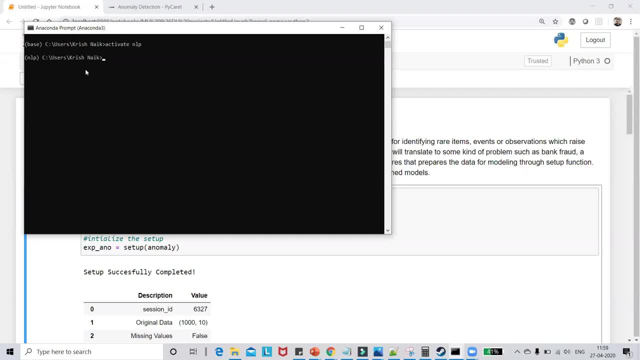 a new environment And if you have been seeing my videos from many days, right, I usually, whenever I upload any- you know project sessions- I usually create a new environment itself And I think you should know how to create a new environment if you're already learning. 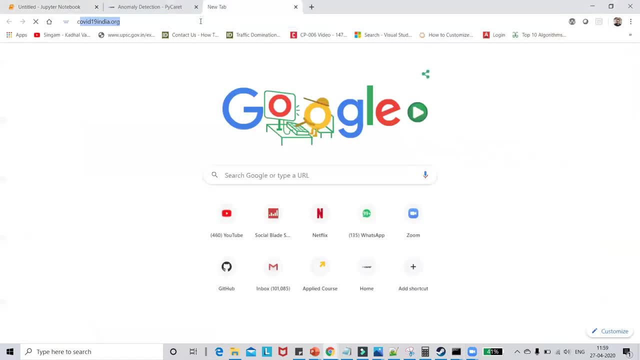 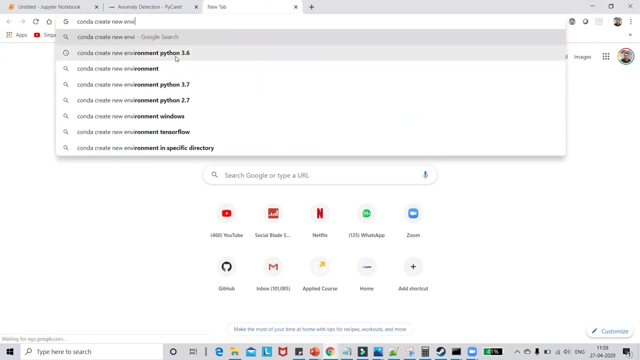 from it, right? Otherwise, just go and see search in the Google saying that Conda, create new environment, right. Just go and search in this particular thing- environment Python.3, 3.6,. you'll be getting a command and by that you'll be able to do it. So once you do it, 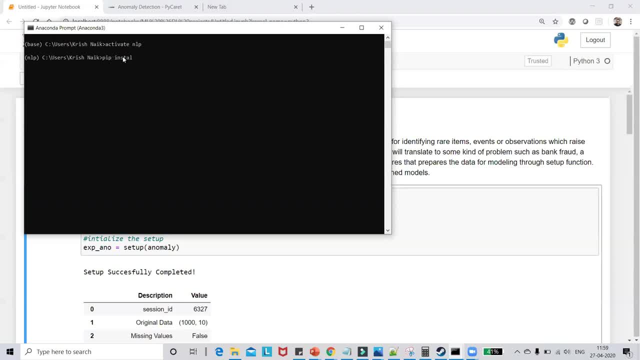 you just have to write pip- install PyCaret. right, That's it. you just have to type this particular command and automatically the installation of PyCaret will happen. right Now, many of you will be facing this issues, probably because that is because you are actually installing. 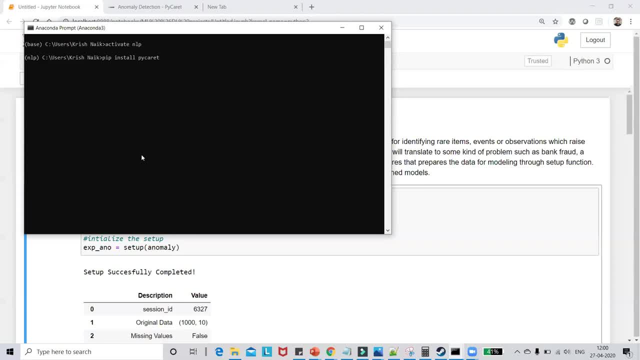 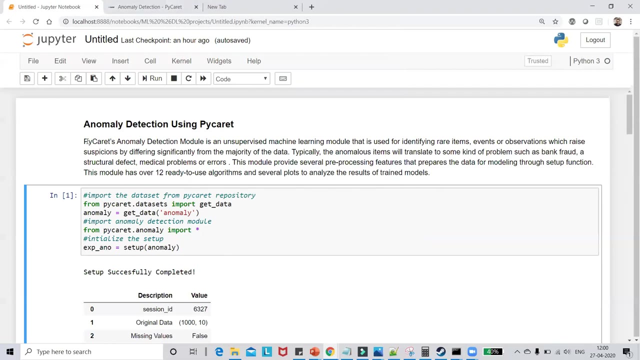 it in your base environment. Don't do that. create a new environment and install the PyCaret library over there- And this is an amazing open source library, guys- because it will definitely help you to do your work a little bit faster when compared to the previous techniques that we used to do. right now, Let us go ahead and 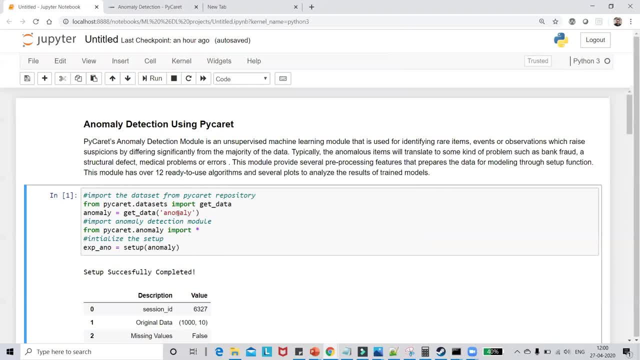 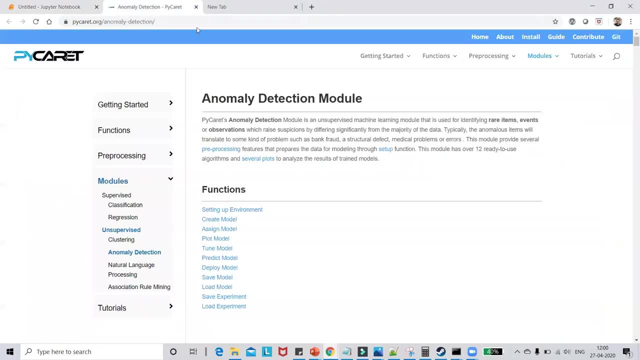 try to start what we are actually doing Now. we have a data set which is called as anomaly. Now, in this particular anomaly data set, guys, I'll just show you the data set of what it is And anytime, if you want to know about the description, you can actually go into. 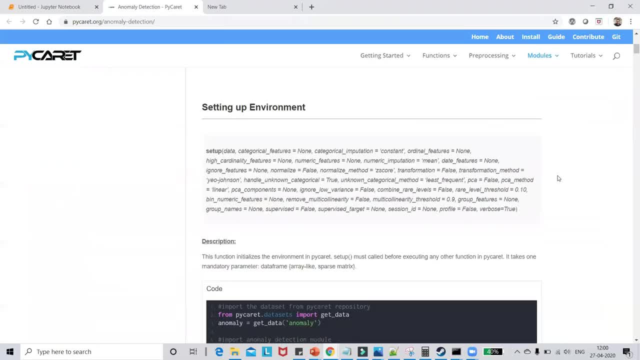 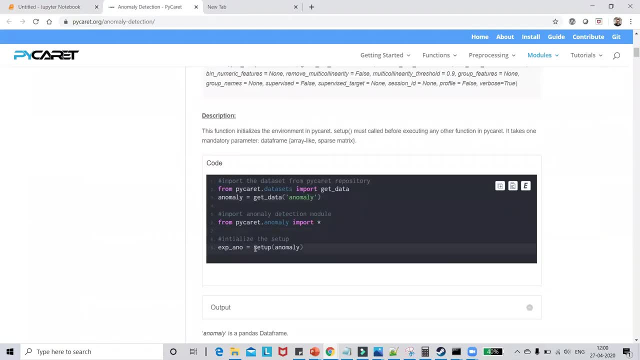 this particular page And again, the link will be given in the description of this particular video. So the first time we need to set up the environment, which we have already done Now. after that there is a function which is called a setup Okay, And initially you will try to import. 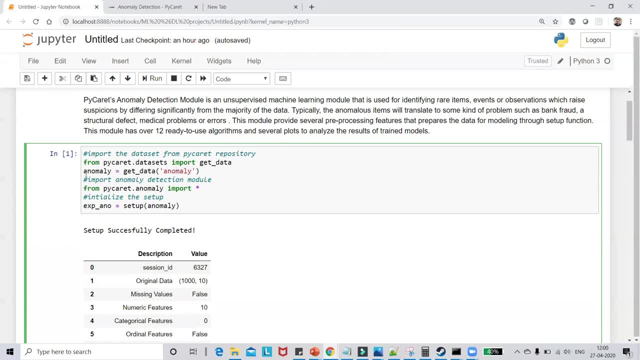 the data set because there is an inbuilt data set which is called an anomaly inside PyCaret. So, in order to call that data set, what I'm going to do is that I'm going to write from PyCaret dot datasets: import: get underscore data. anomaly is equal to get underscore data. 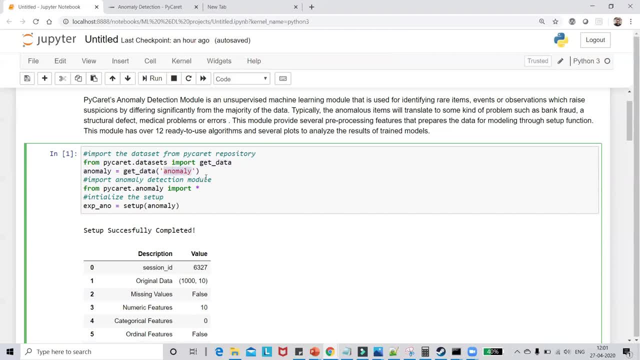 And in the in the you know parameter, I'm giving it as anomaly. this is the data set name, right? So after that, whenever you want to apply a classification algorithm or regression algorithm, you need to import from PyCaret dot classification import star or, if you are trying to do it, 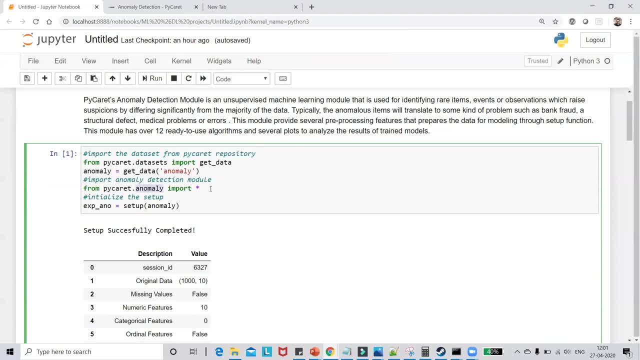 with respect to regression, you'd have to write PyCaret dot- regression- import star. Now, in this particular case, it is anomaly. Anomaly is a different module that is created by Python, So I'm going to write from PyCaret dot: anomaly- import star. Okay, And initially, 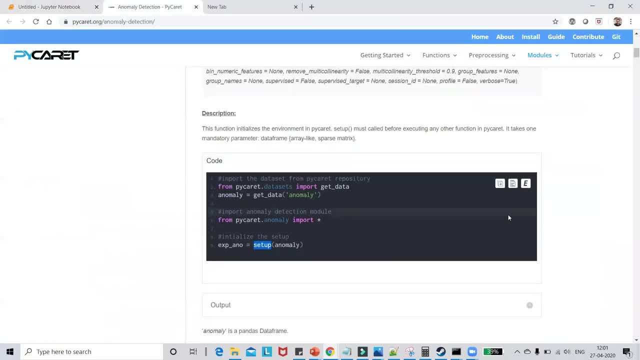 we do this particular setup. Now, what does this set up mean? Let's, let's go ahead and do it. Let's go ahead and do it. Let's, let's go to this particular what this setup function does In setup, it takes a. 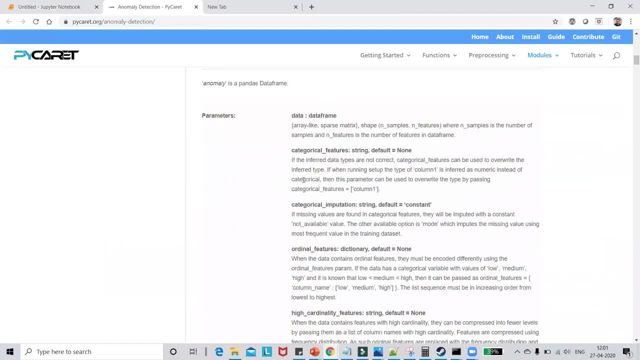 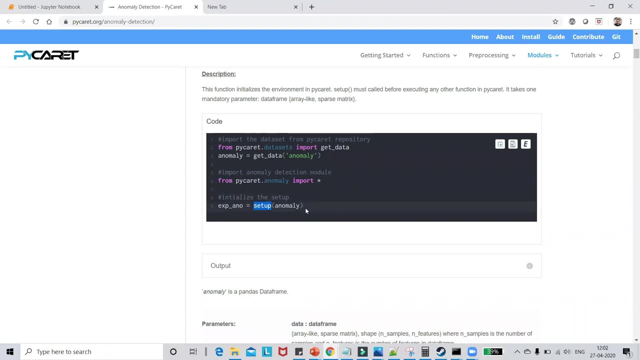 lot of parameters. First is the data, which is in the form of data frame. All the feature engineering steps can be actually done by providing just the parameters inside this particular setup. Now what? what kind of feature engineering starts, If you want to handle? 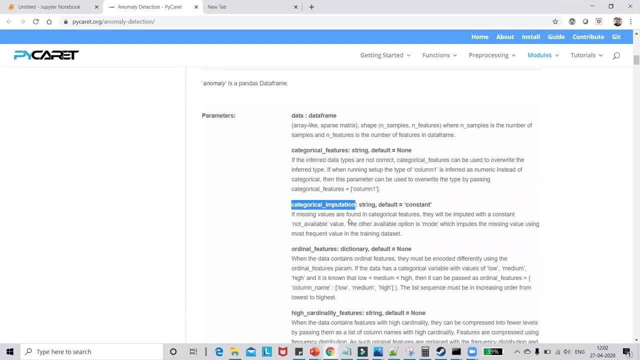 category features. right, If you want to handle category imputation- suppose there are a lot of NAND values in a category feature- then you have to follow some imputation technique. You can basically, you know, put this particular set of parameters into the set of parameters. 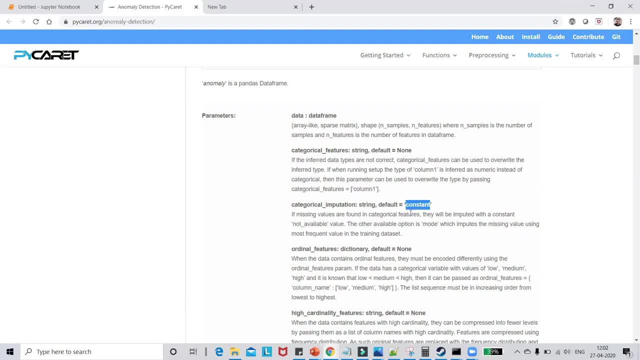 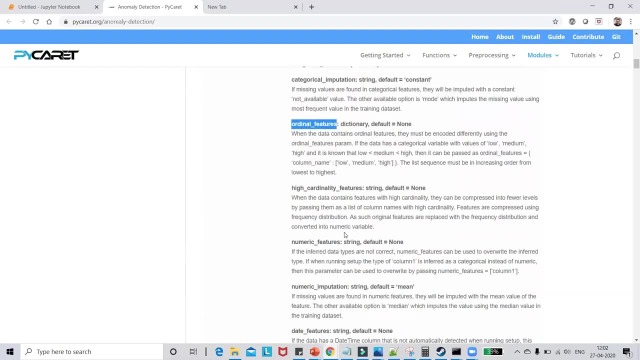 Okay, If you want to handle a particular value by default, it will be constant. That basically means if it finds a NAND value, it will replace it with a new constant category feature: right, It also handles ordinary features, high cardinality features, numeric features- you know numeric. 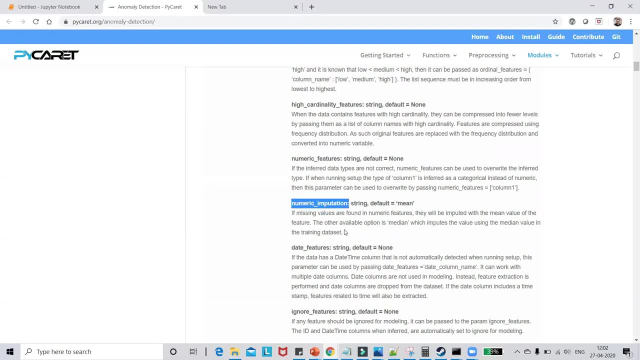 imputation. So if you, if there is a numerical column and if there are a lot of NAND values, by default it is going to use this mean technique. You can also change it to median and mode. It is up to you And again, for that you just have to see the data that you actually 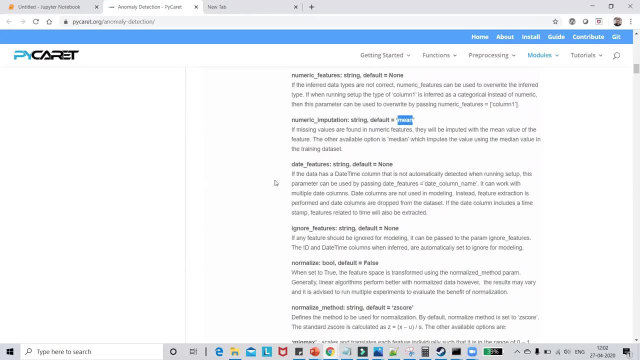 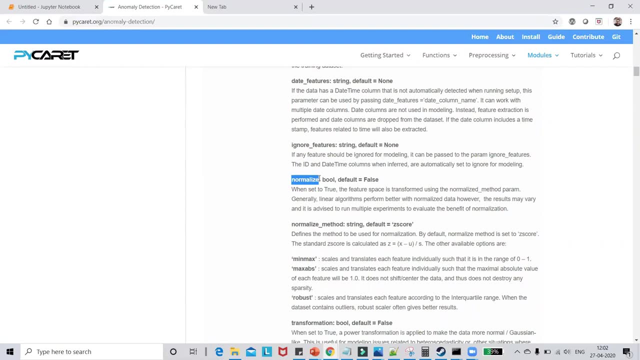 have and how the data distribution is Okay. Then you also have something like normalize, So normalize. you know that in case of if I take an example of k-means clustering, or if I take an example of linear regression, logistic regression, at that time I have to set this normalized value as true By default. 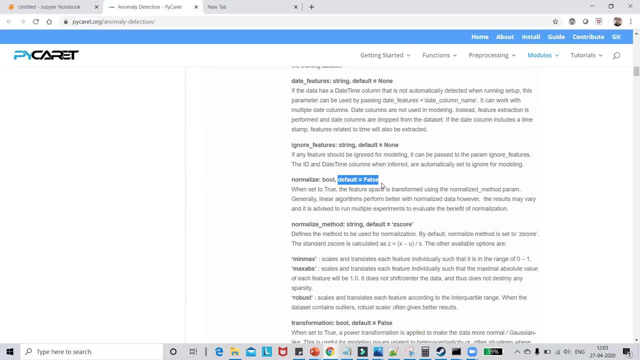 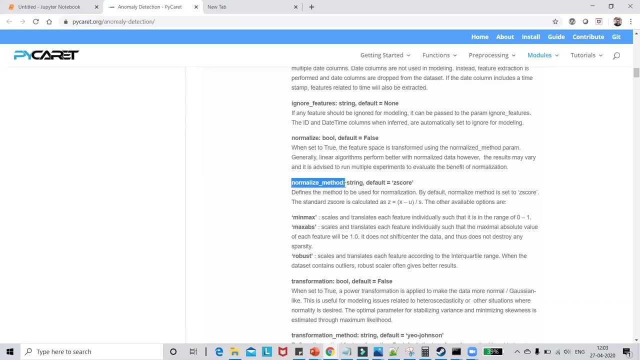 it is actually set to false, So it is going to scale down those features. And there is also like a normalized method. You know, once we set the normalize is equal to true, we also need to set this particular method, And this particular method by default is z-subtracted. 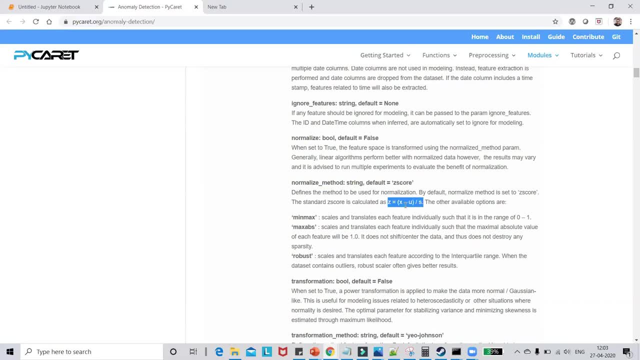 Okay, And you know the z-score formula is nothing but x minus mu. Mu is basically the mean divided by standard deviation. I hope I've already uploaded these videos in my stats playlist. You can actually go and watch. So this particular normalization method when it is scaling down. 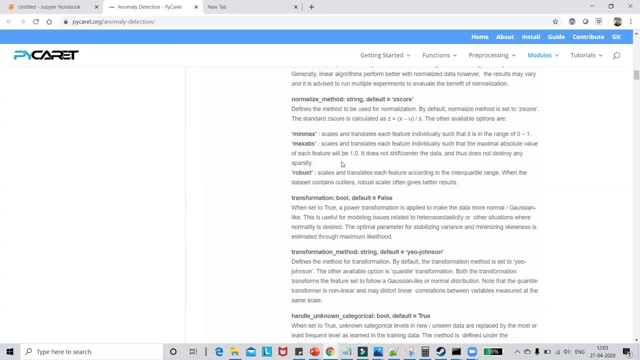 all the features. it is going to use this z-score technique. Other than that, you can also set, with respect to min-max, max-ebs, robust, and many more techniques are there. as we all know right, Min-max actually converts your values between zero to one and other. 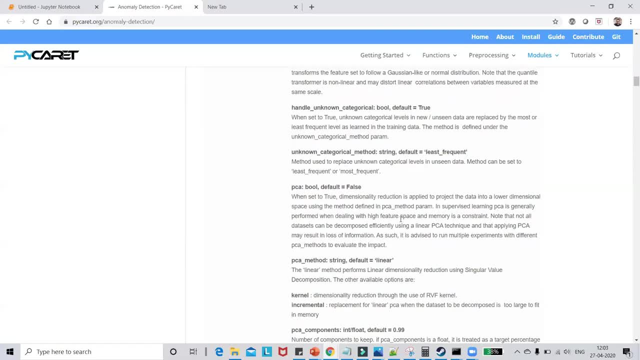 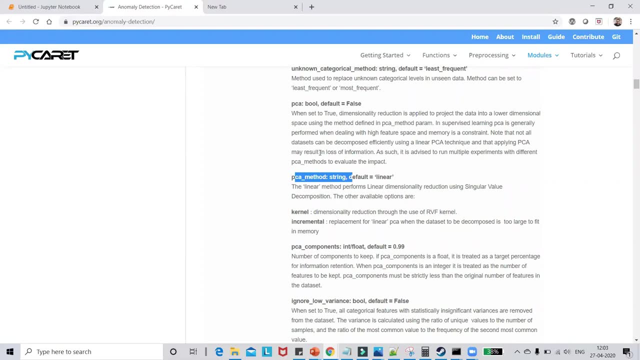 things are also present. Okay Now, with respect to this, you also have a PCA technique, whether you want to implement a principal component analysis that is, dimension reduction, And by default over here it is linear, So linear. it usually performs this linear dimensionality reduction, If you know. 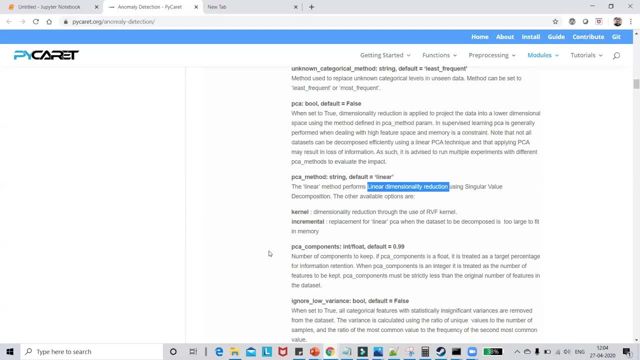 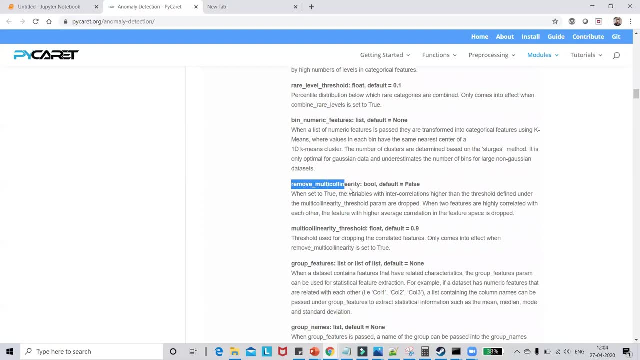 this. I think you should be knowing this, because it is pretty much important Apart from that, how many PCA underscore components you want, and a lot of more parameters are there. Okay, This is a wonderful parameter. Remove multicollinearity. I'd like to talk a little bit about multicollinearity. 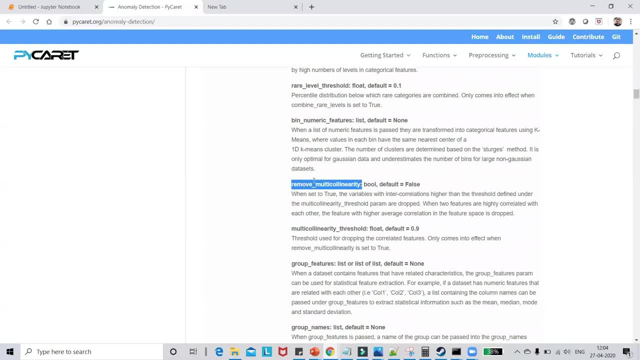 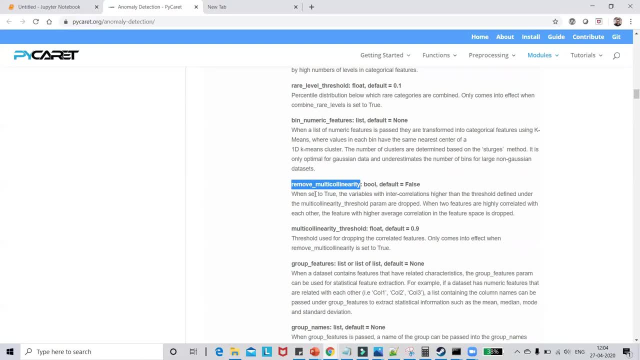 actually help you to do the feature selection. If two features have a huge view, I mean if the two features are more similar, at that time what will happen? the correlation will be quite high, right? So in that particular case, those two are actually co-linear with each other, So we'll. 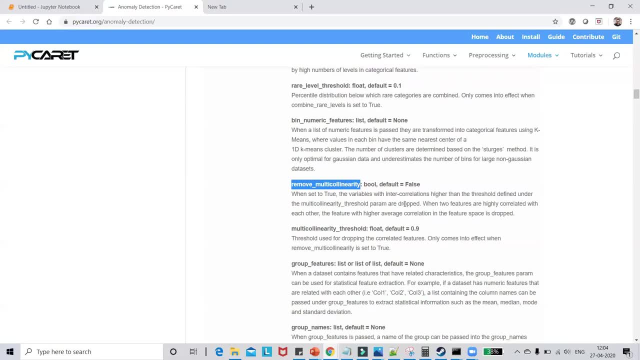 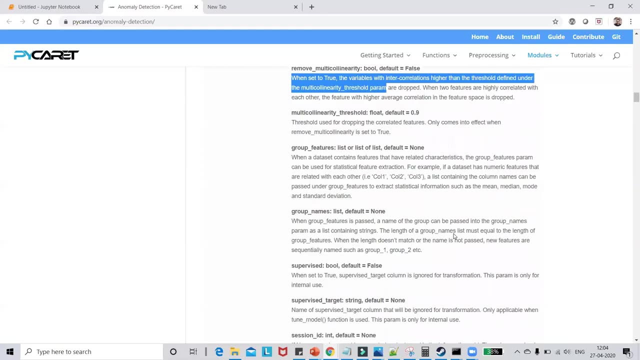 try to remove those kinds of features which are actually highly correlated, right? So by default, we'll be. by default, it's set to false, but we'll try to set to true in order to solve this particular problem. and again, you can actually explore. there's so many parameters as such. so right now, by default. 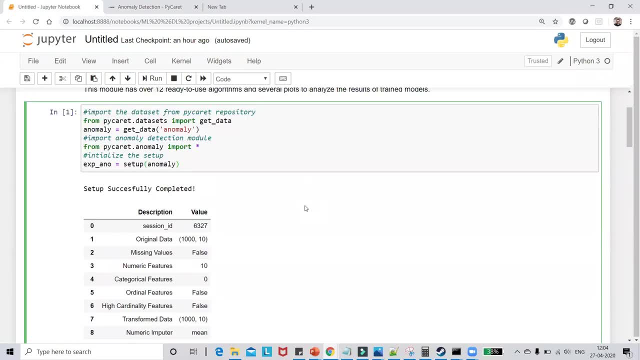 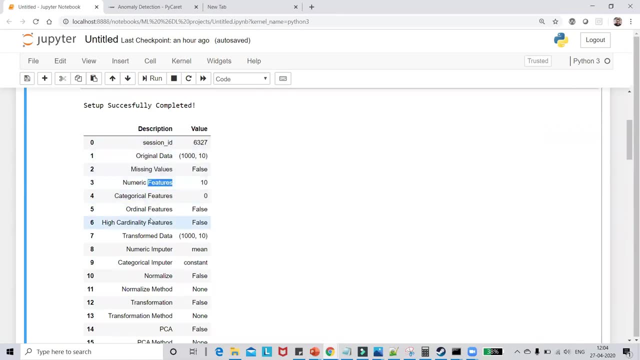 whatever is the default value, i'm trying to do it and you'll be able to see that you'll be getting all these kind of descriptions. you'll be able to see that what all values we have been set for missing value, numerical features, original features, false, true, false, true. is there now, once it is. 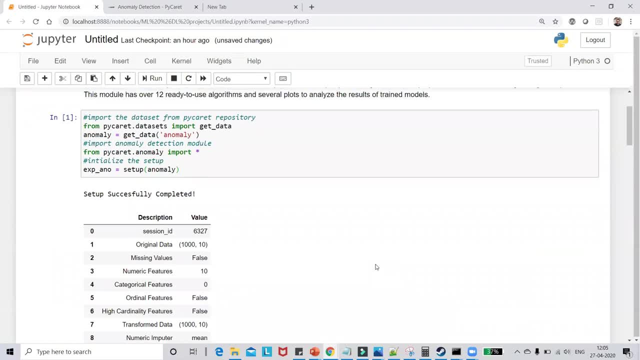 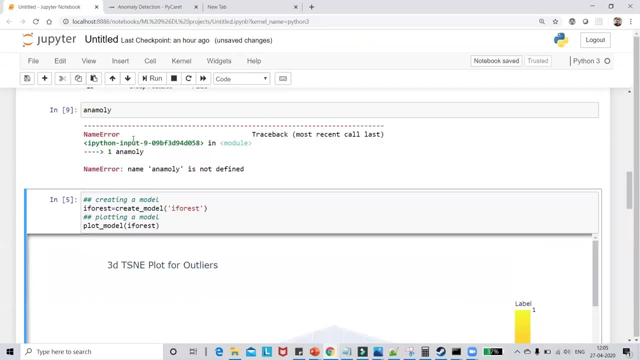 executed. i'll just go and what i'm going to do is that i'm going to just go and see this particular data set which is anomaly and again i told you guys, this particular technique is an unsupervised machine learning technique. okay, i'm just getting an error. oh, sorry, spelling mistake. with respect, 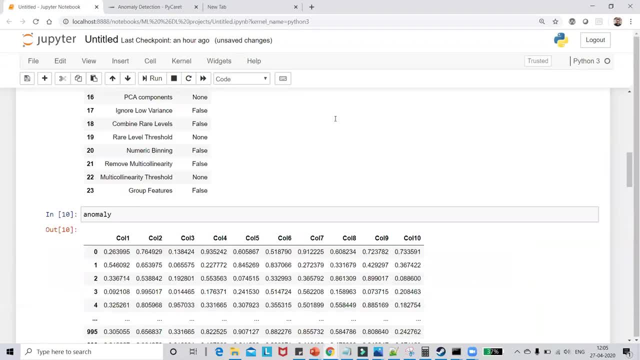 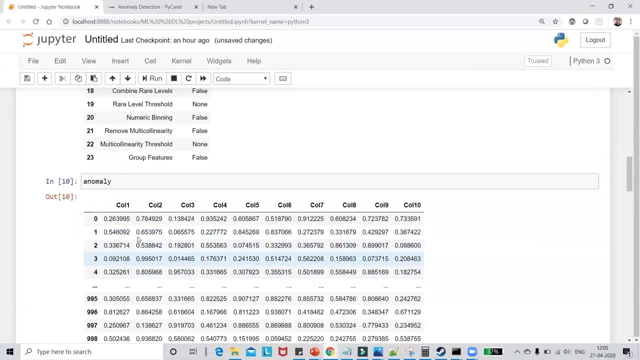 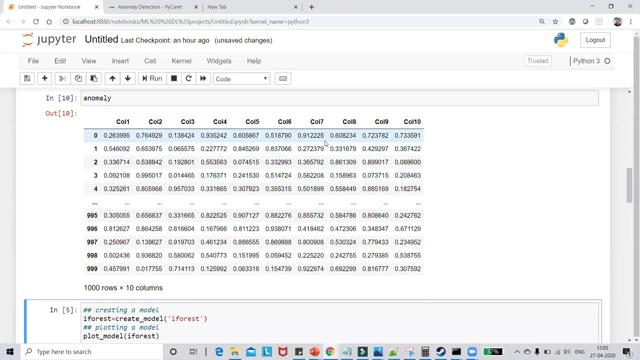 to anomaly, probably. i think i've made a no, that's fine. now this is: this is my data set. okay, and this is just an anomaly data set. you have a lot of values with respect to 10 columns and out of this we need to find out which record is. uh, you know it's an anomaly, it's kind of like a fraud data. 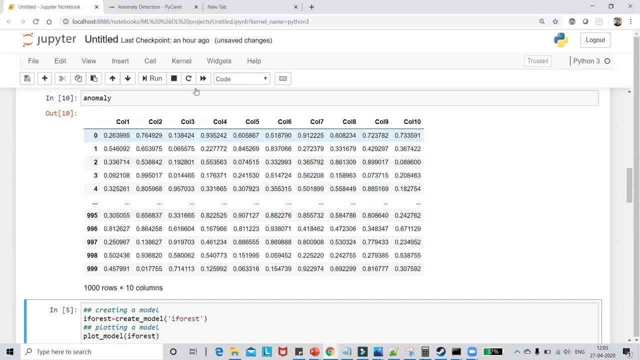 set. it is a fraud data set. it is a fraud data set. it's a fraud data set. it is a fraud data set. it is that is actually present when compared to the whole group of data. right by just seeing this, we cannot definitely see what, which one, which record is actually fraud. so let's go ahead and 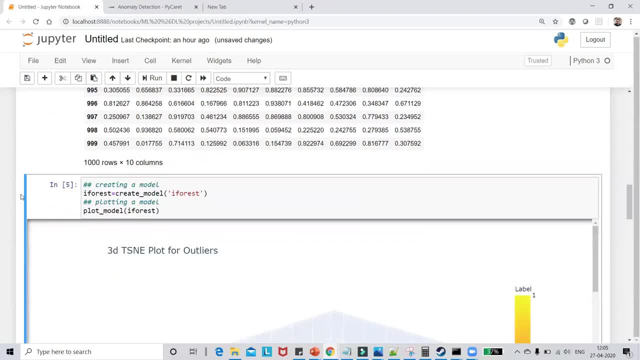 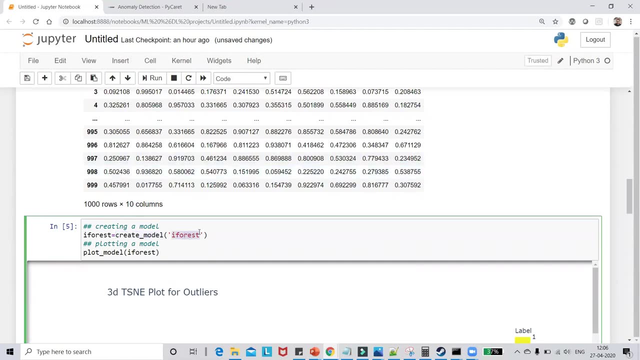 try to see this and how to solve it. okay now, the next thing is that we have an inbuilt function inside this anomaly which is called as create model, and the type of technique i'm going to use is called as iforest. now, from where did i get all this particular parameters? if you go over here, 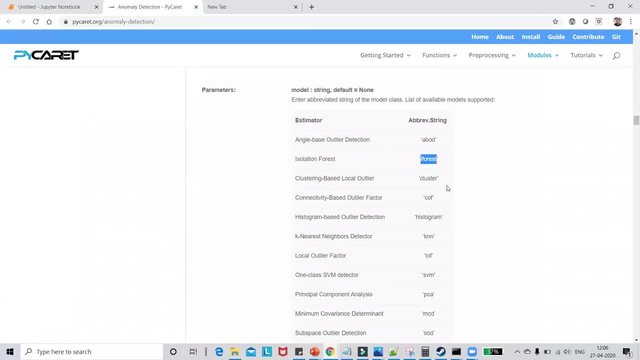 guys, when we're creating the model. there are a lot of techniques like iforest, cluster, knn histograms, histogram based outlier detection, clustering based low local outlier, connectivity based local outlier- sorry, outlier factor- isolation, forest. a lot of techniques are there, and probably this many techniques you may also not be knowing with respect to anomaly detection, right, so there are. 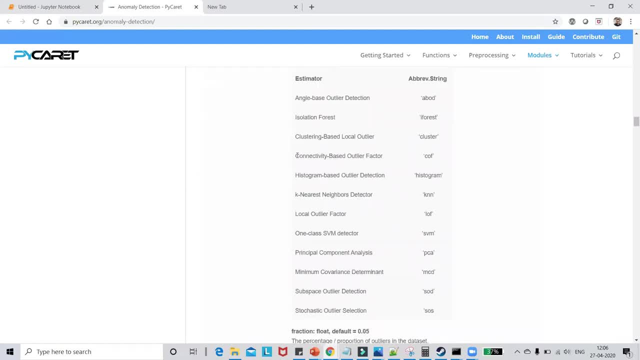 a lot of things, uh, that we probably do not know with respect to outlier detection, but this particular library gives you all the particular option, right, so you can select one of them. uh, just try with isolation forest, and then again we can also compare with other by seeing the visualization diagram. so, isolation forest. what i can also do is 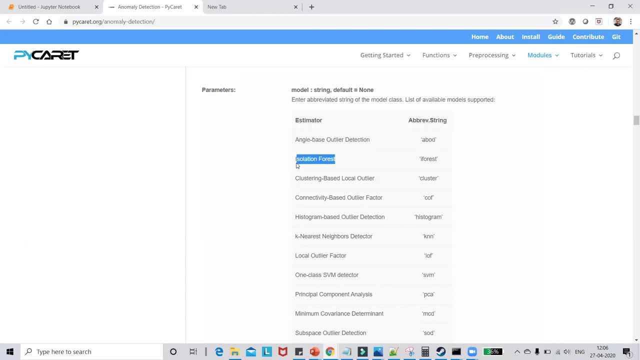 that i can go and see. i can actually go and see for isolation, forest and k nearest neighbor and then i can actually compare like how many have been grouped as zeros, how many group have grouped as one right. that will basically indicate whether it is a fraud or not, right? so right now i'm just 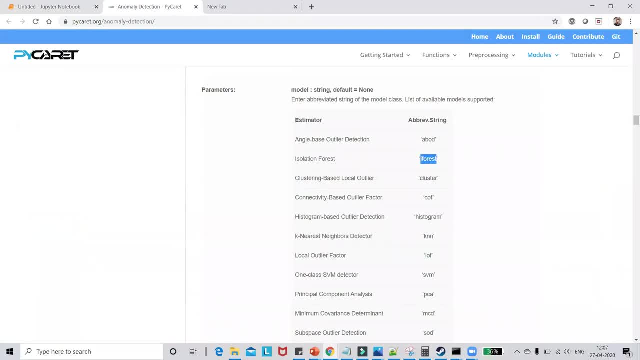 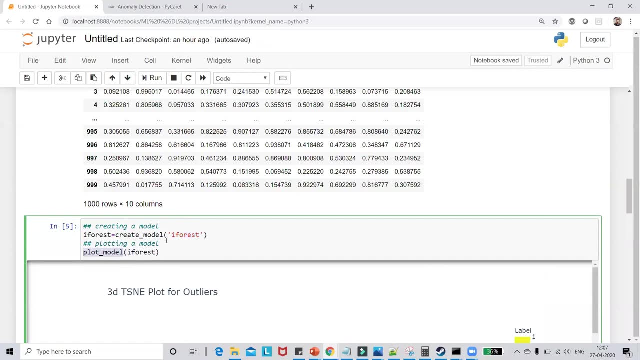 using iforest. i'll be using. i'll just copy this same term i forest and paste it over here. then you can see that i will be using plot underscore model, which is again an inbuilt function inside pi caret, and here i'm just going to give this particular 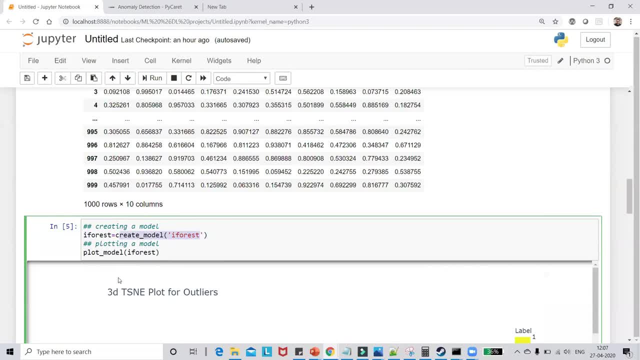 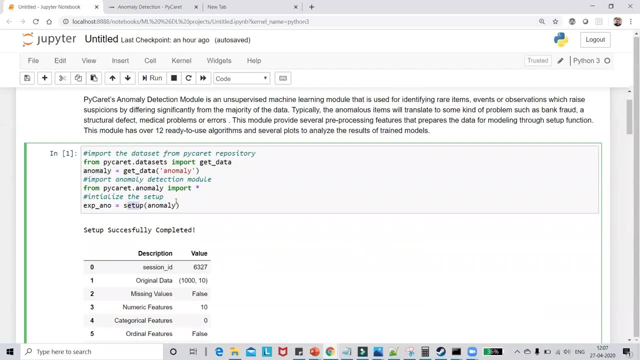 model i forest. now, when i do create model with i forest, this internally is going to take this particular data that is called as anomaly. right, because i have actually made this setup over here. right, because of this setup, this is this variable is getting created and this, in turn, is actually: 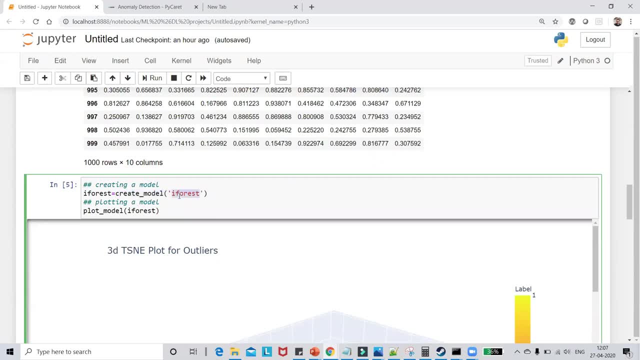 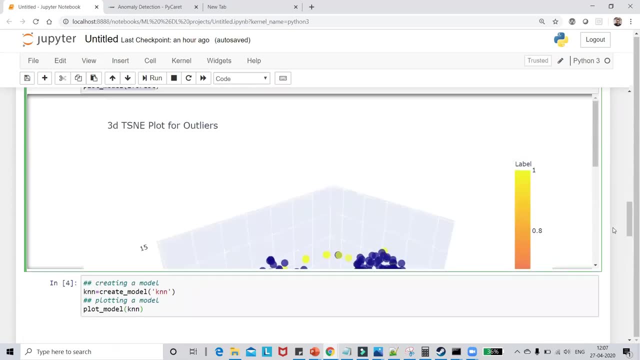 taken by this particular uh library, that is i forest, and paste it over here and then i'm just so i'll target that property, that is i forest, as the data right. so when i do create underscore model and when i do plot underscore model- i forest, i am going to see a visualization diagram, right? 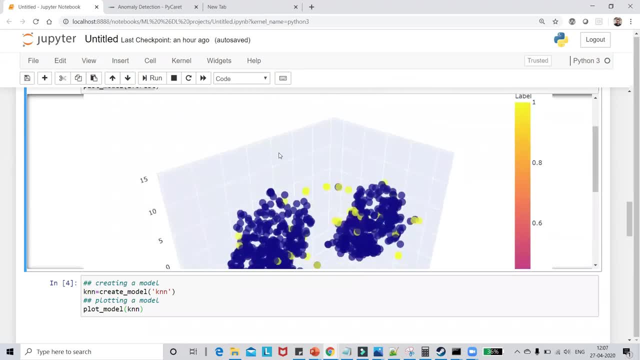 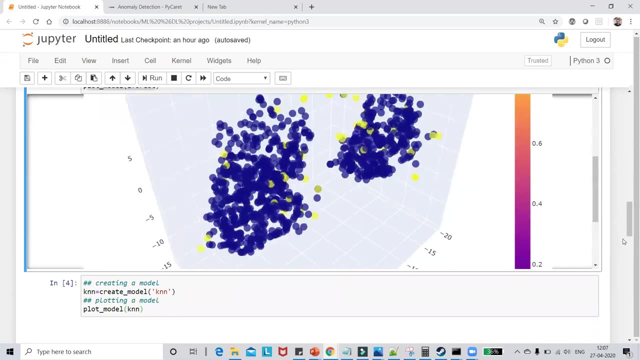 now, as you know that we had around, you know, 10 features over here, right? uh, and trust me, guys, to just create a three-dimensional diagram by using python or other libraries like cbonnet is a very difficult task. now, this yellow points, right, yellow points that you see. 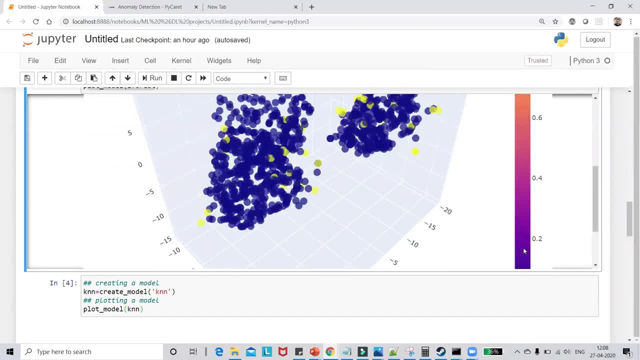 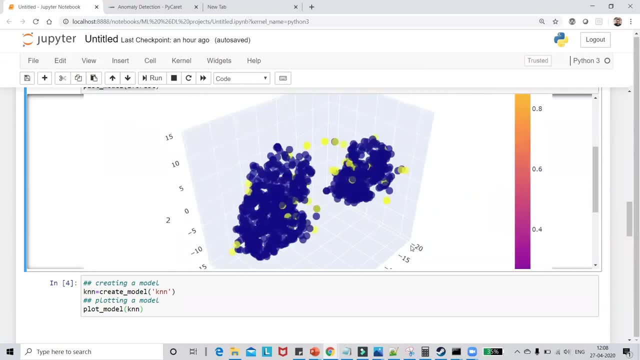 there are two type categories: and zero right. this one basically indicates that it is a fraudulent data- okay, and zeros basically indicate that it is not a fraudulent data. so obviously, in our case, you can see that there are a lot of non fraudulent data, whereas there are very less number of fraudulent data, like this yellow, yellow points that you 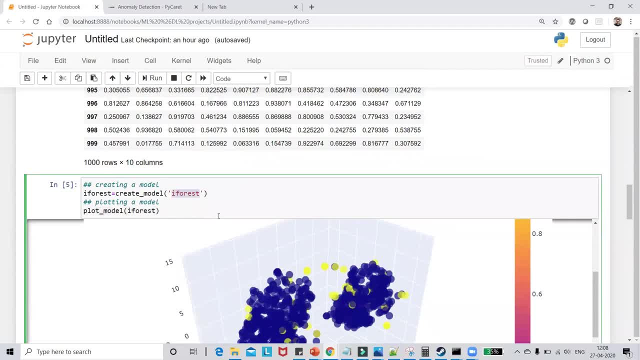 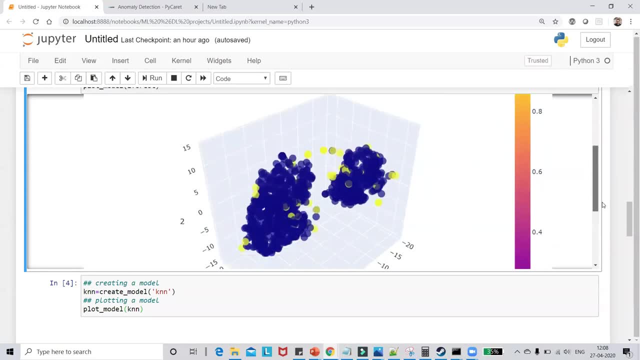 actually see, and here we are using a technique called as isolation: forest right amazing diagram. you can see that clearly, it is visible in a proper way and it looks amazing. with respect to this particular diagram that you see on the right hand side, which actually denotes the color indication, now you can. 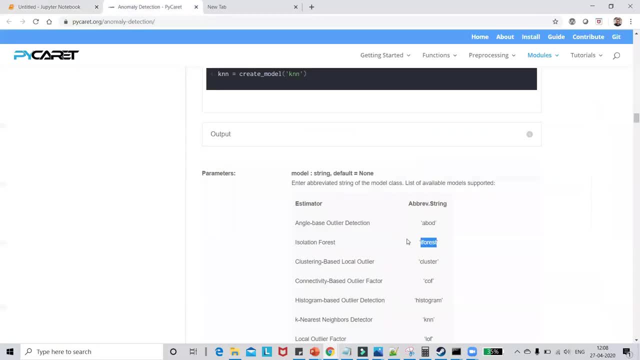 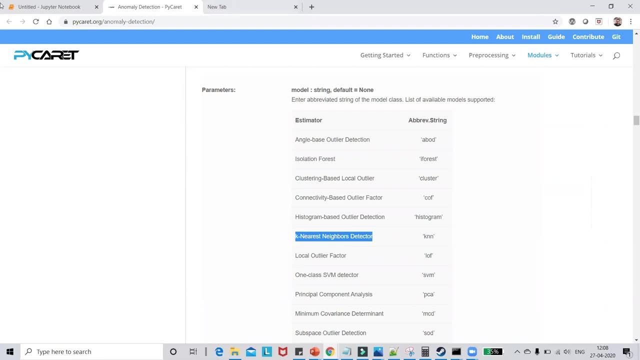 also try with KNN. KNN- if you see over here- that's I can in- is also one parameter which we can actually use for anomaly detection, that is K nearest neighbor detector. now what I'm going to do is that with respect to KNN, you know, 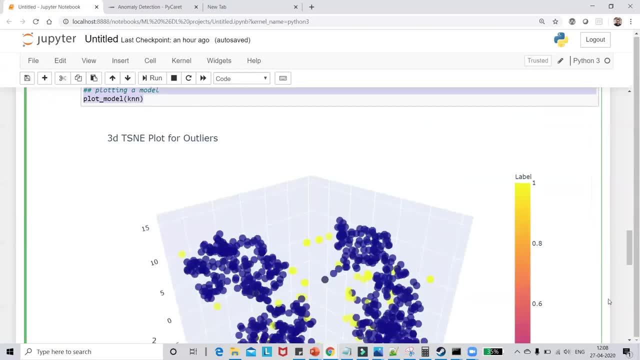 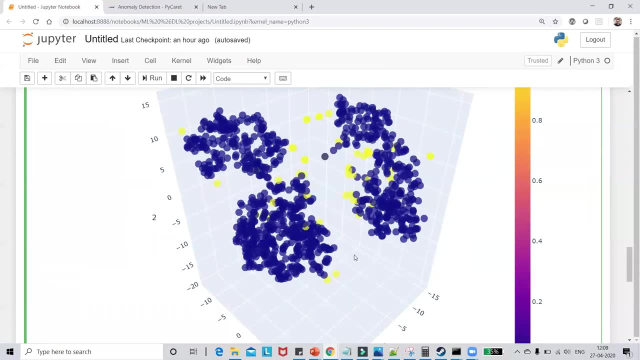 if I try to execute the same thing. right, you can see now this is how my diagram looks like. and again, you can clearly see over here this particular points, which is treated as you know the fraud detector, is quite far away from the similar points that we. that is actually present over here. so these all are my good points. these are: 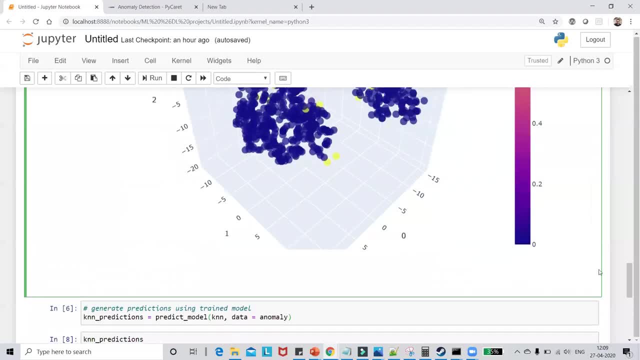 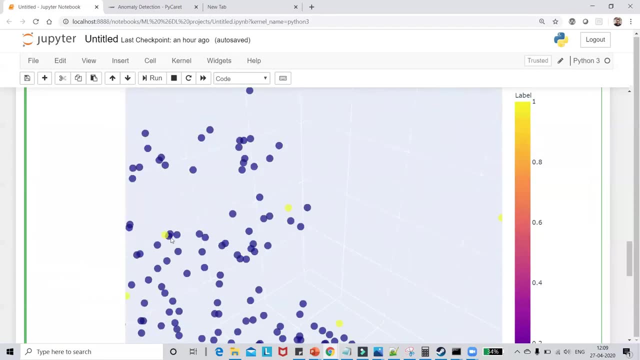 my bad points right. so again, I always remember the bad points will be actually very, very best then. I can also use that same KNN model for this. if I zoom in, this is how my data looks like and you can see a wonderful 3d diagram right and. 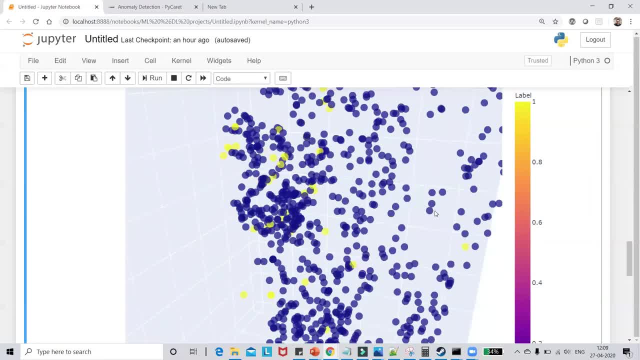 you can see there are no problems with the club. you can see all these lines that I have created and I also, I have the same problems with the club and I also, I have the same problem with the club. I mean, I don't know what kind of 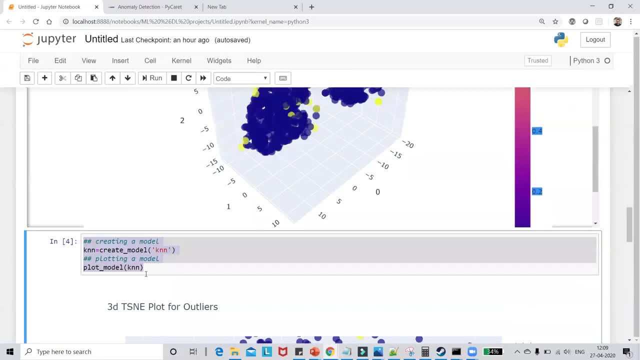 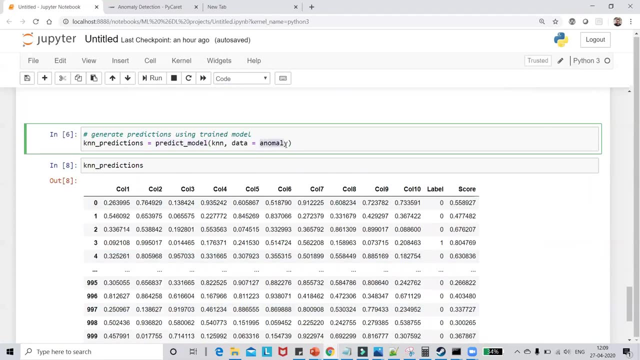 problems do I have is not that I know what's going on, what's going on, what's happening. but okay, so let's go up and you can see that I have created this particular model, KNN, and now I'm just going to do predict underscore model and 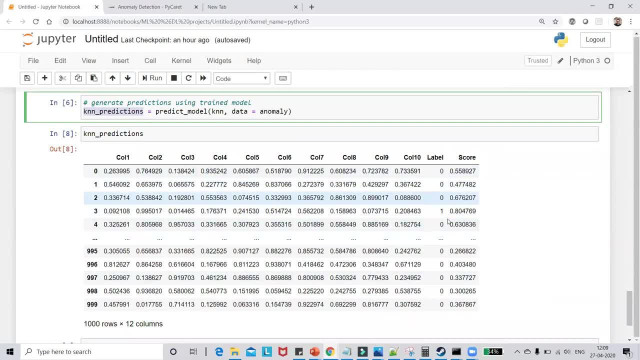 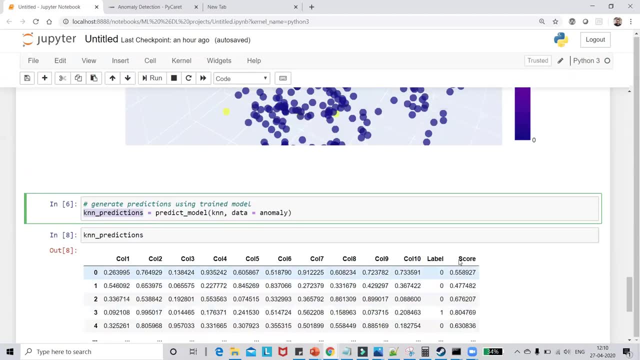 I'm giving the same data. normally, once I see the K linen prediction, I'll be able to see whether it is assigned to labels zero and one, and remember, one is nothing. This is an amazing way: so quickly, just by writing six lines of code, six to seven lines. 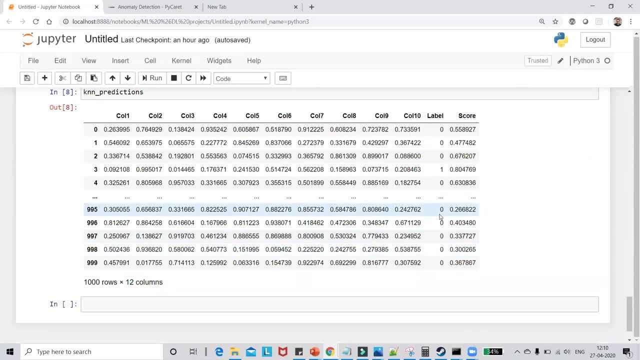 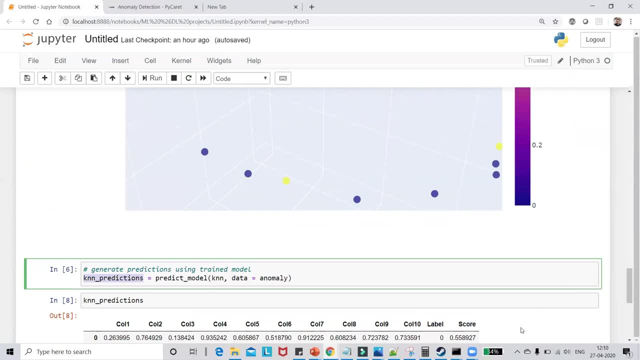 of code, I was able to solve this particular problem, and I even tried this for candle competition guys with respect to credit card anomaly, and the result was again pretty much amazing. Now what you have to do is that just try with other techniques, like local outlier factor. 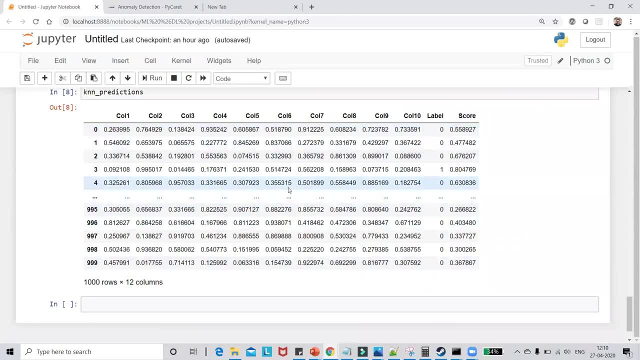 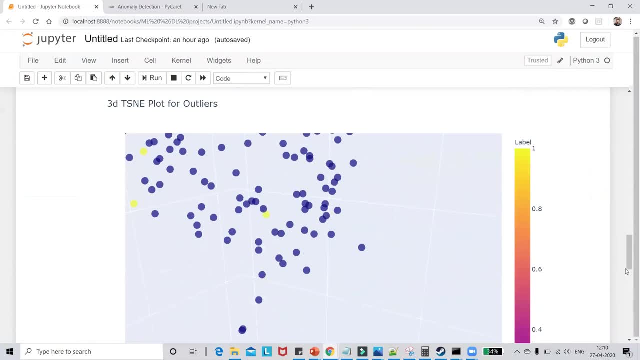 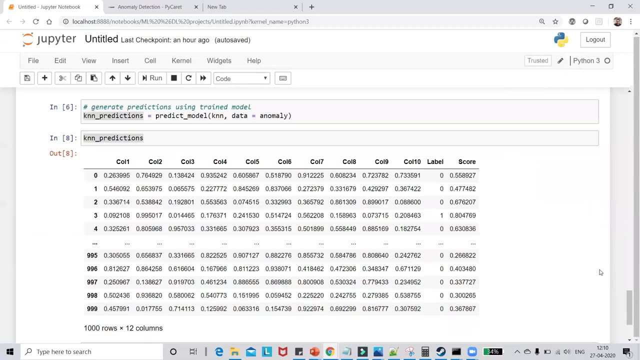 one plus SVM detector and try to compare this label like this KLN prediction. try to compare with whatever prediction that you get with respect to iForest and try to compare. try to find out the confusion matrix. how good it is. Just consider why and why hat, and then you just construct a confusion matrix. 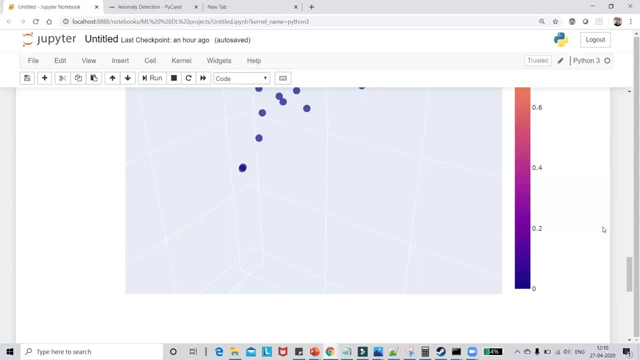 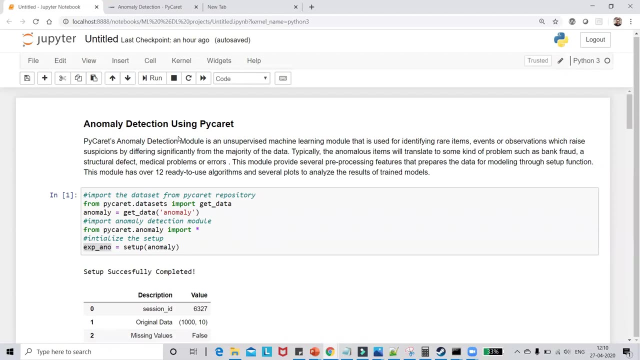 This is a part of the homework that I want to give it to you. In my next video, I'm also going to come up with a clustering problem statement with the help of PyCaret, and I've already created a separate playlist. The playlist link will also be given in the description of this particular video, with 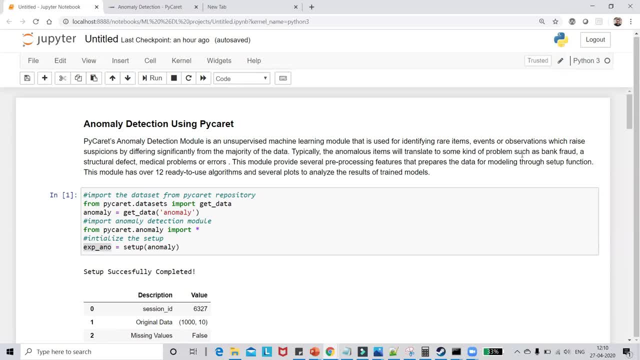 respect to PyCaret. you can actually follow that And yes, this was all about this particular video. Hope you like it. please do subscribe to the channel and in order to subscribe, I'll see you all in the next video. Have a great day. Thanks for watching it all, Bye-bye.